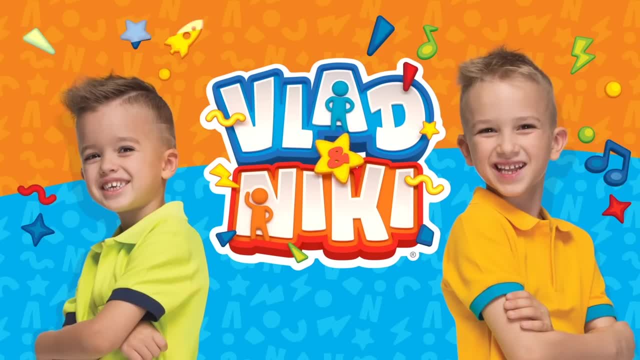 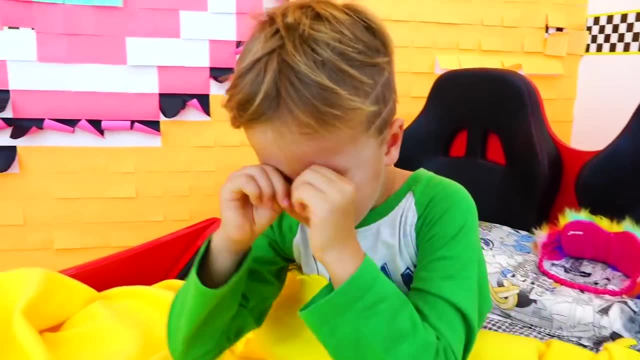 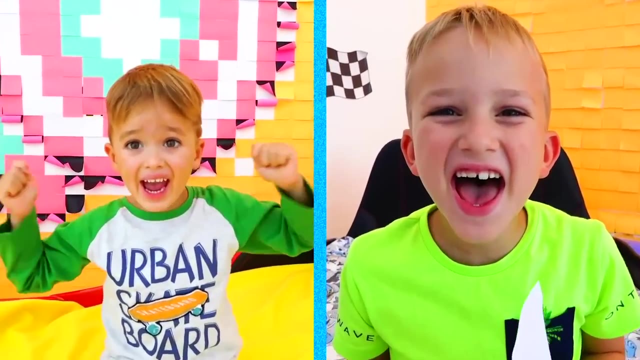 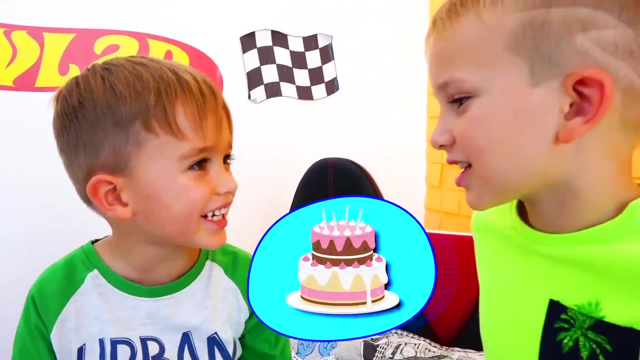 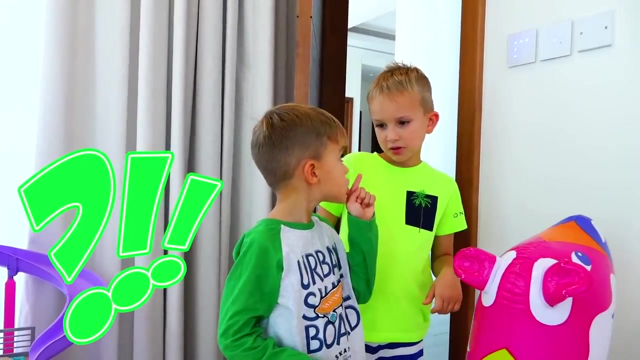 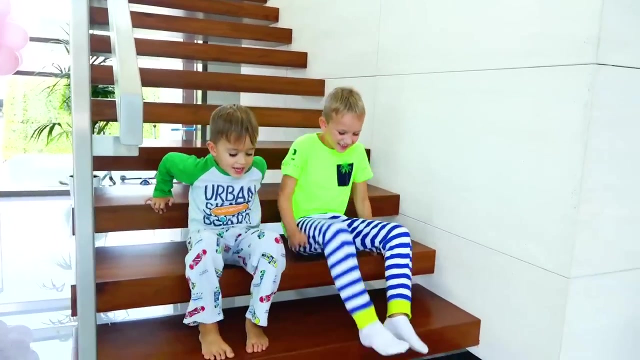 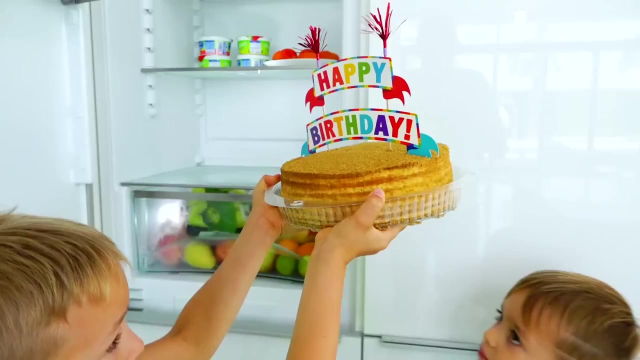 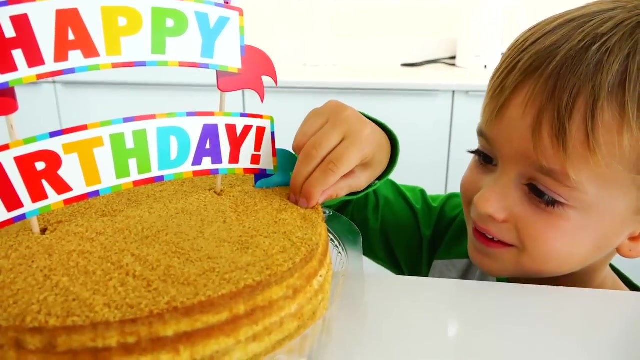 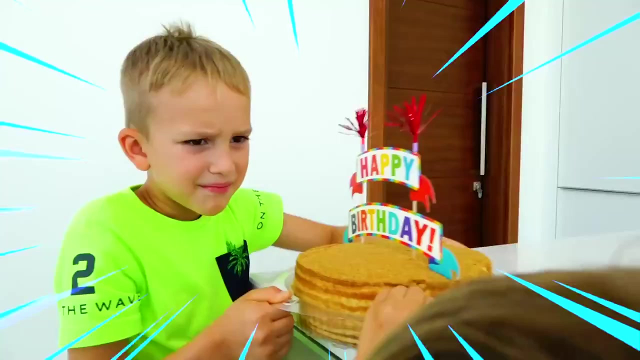 I want a cake. Let's go. Wow, It's Mommy's cake. Happy birthday, Mommy. I want to try. No, no, no, It's Mommy's cake. No, no, no, Why, Why, Why. 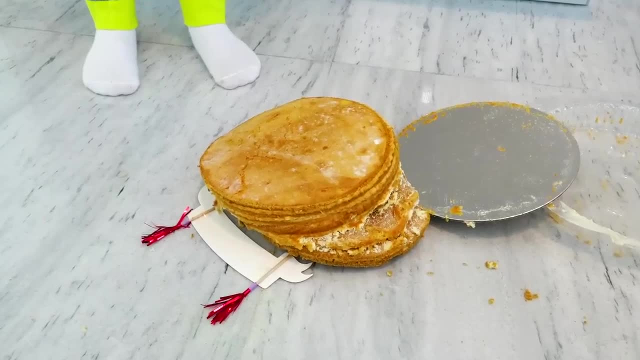 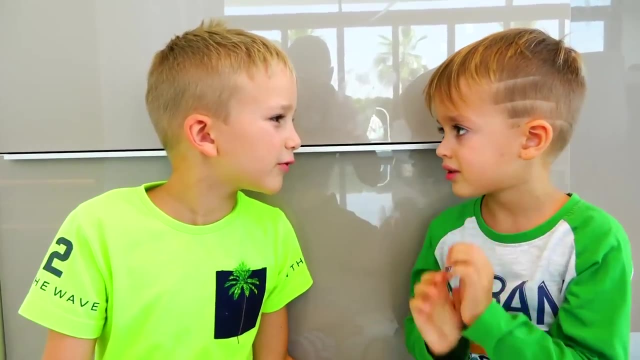 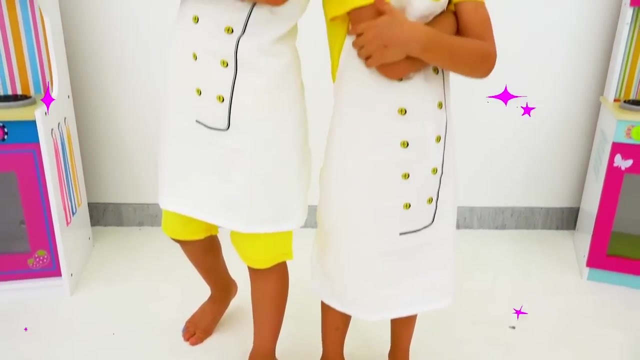 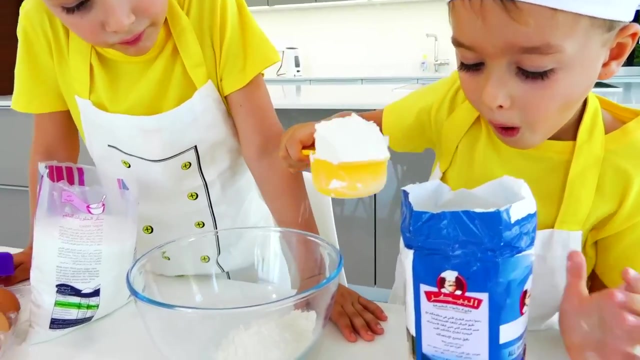 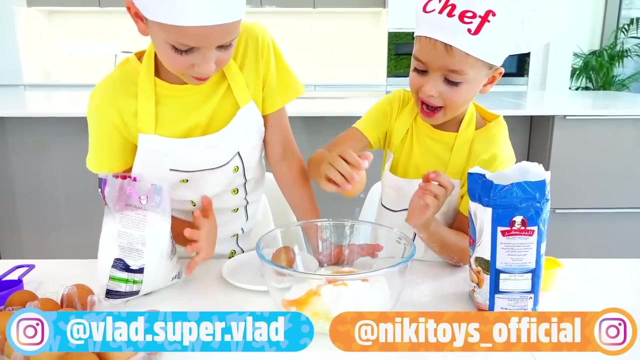 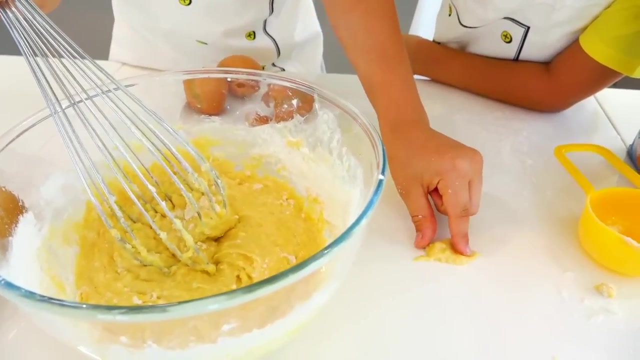 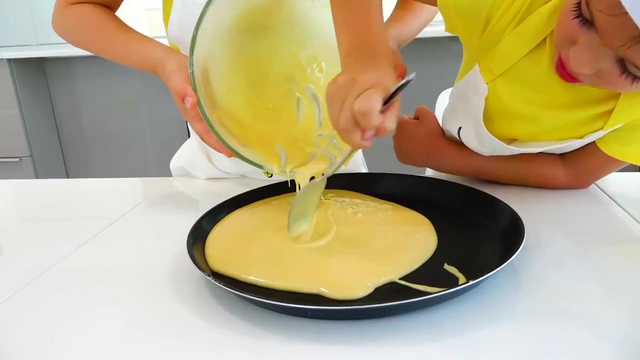 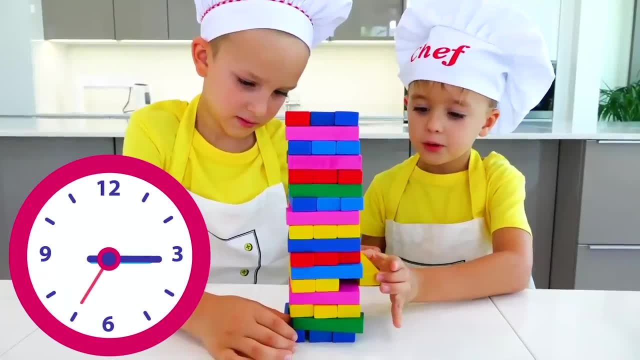 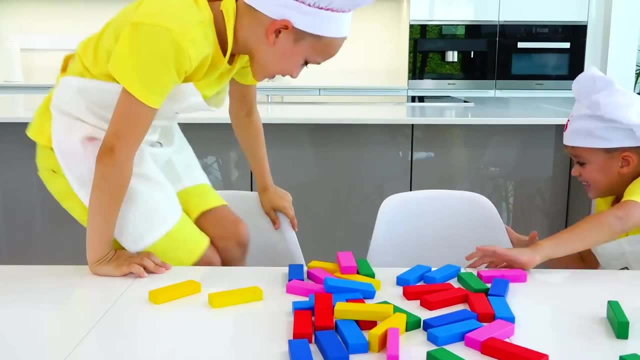 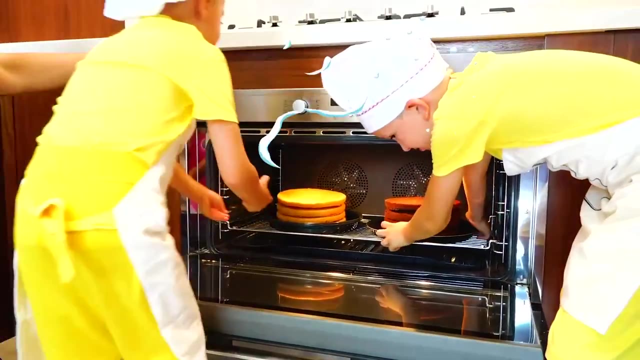 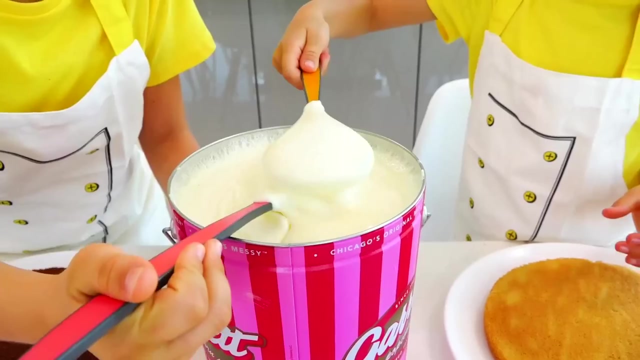 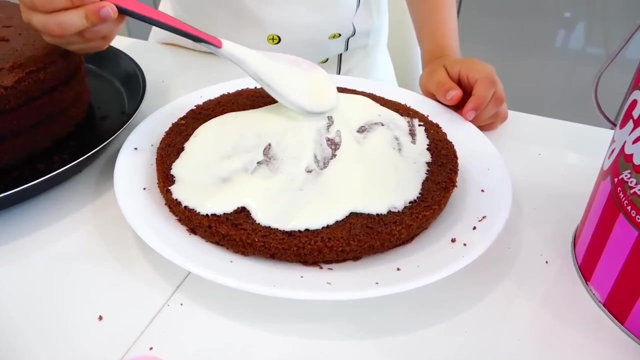 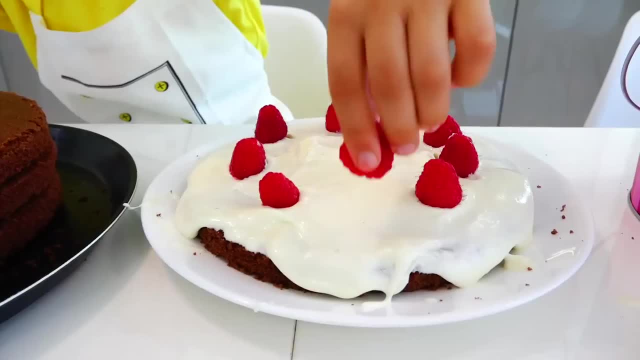 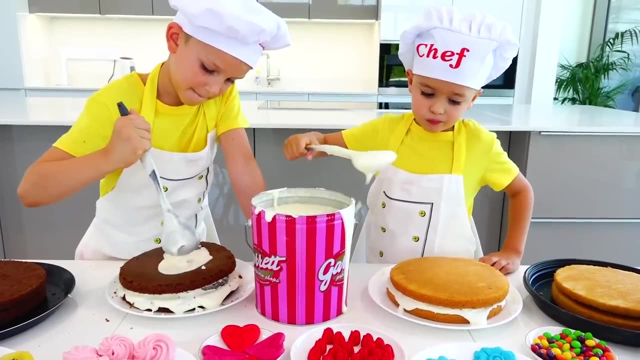 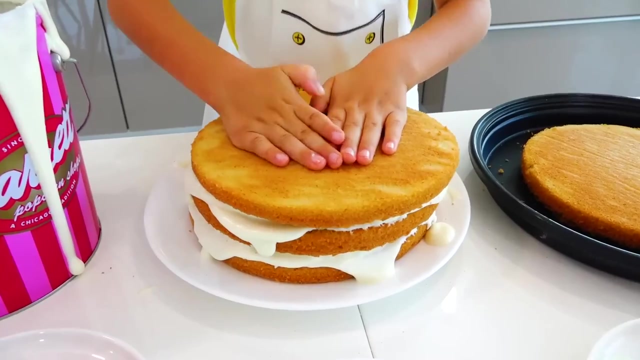 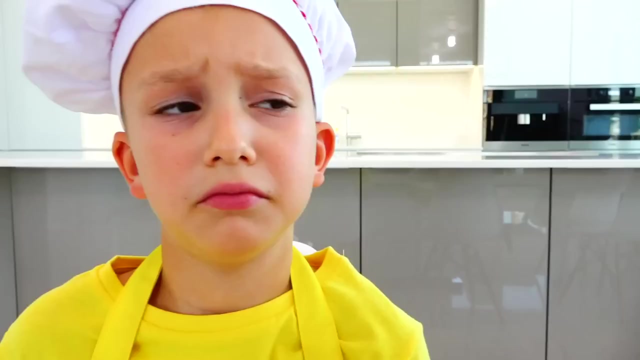 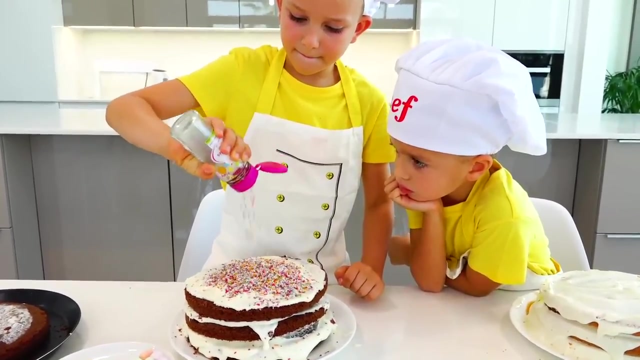 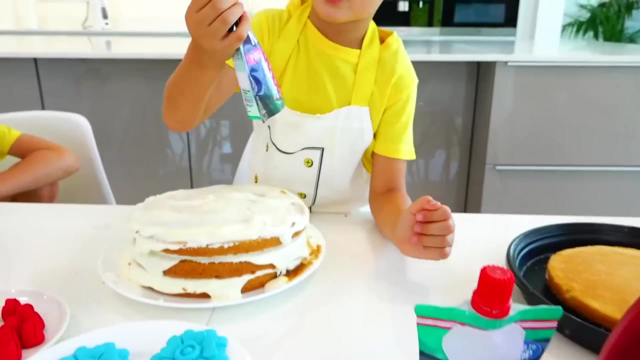 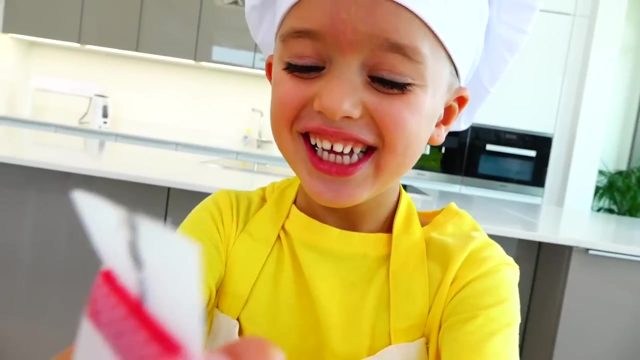 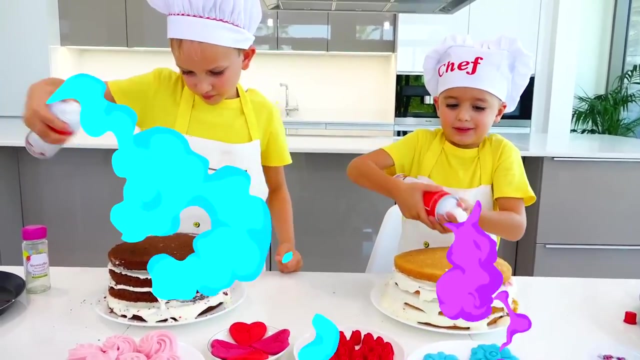 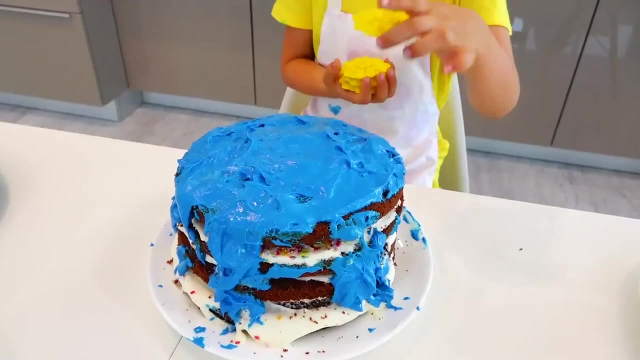 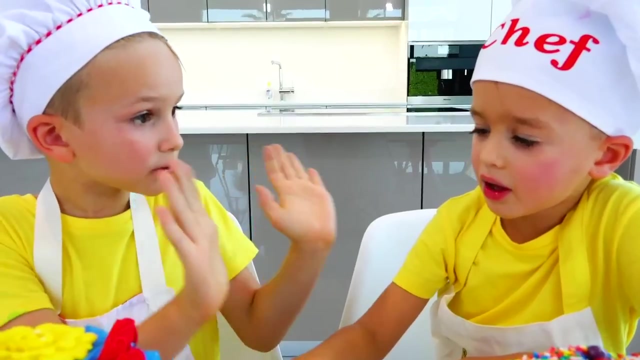 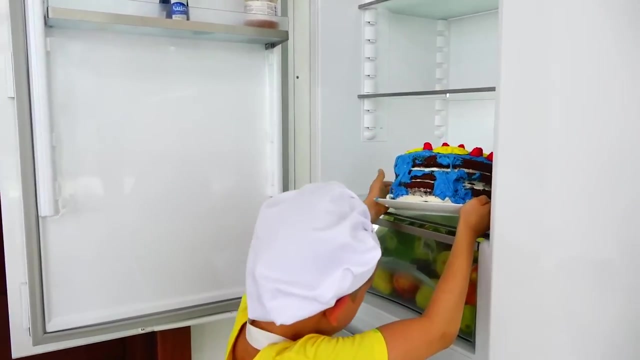 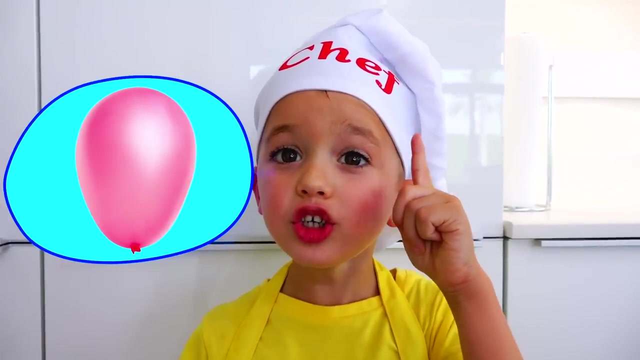 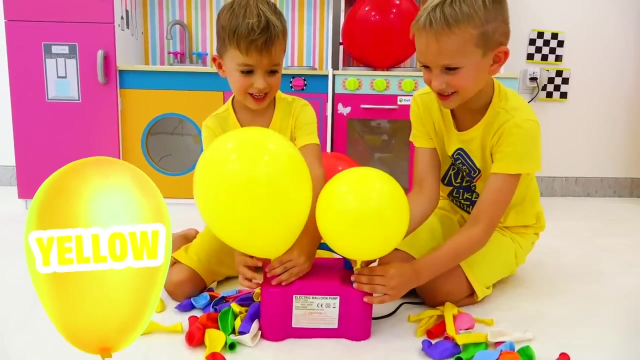 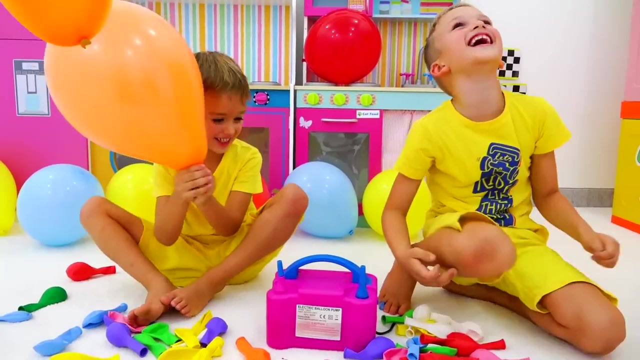 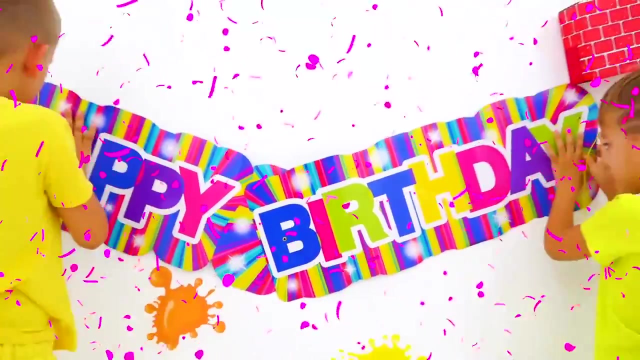 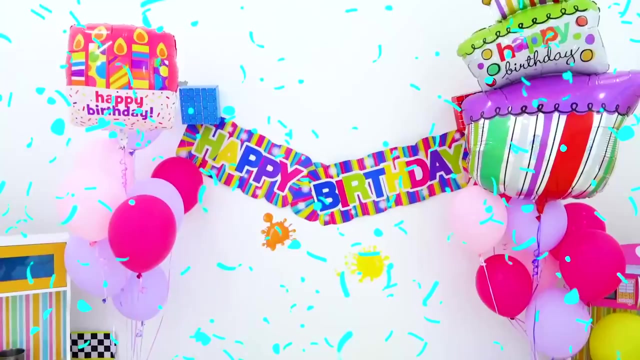 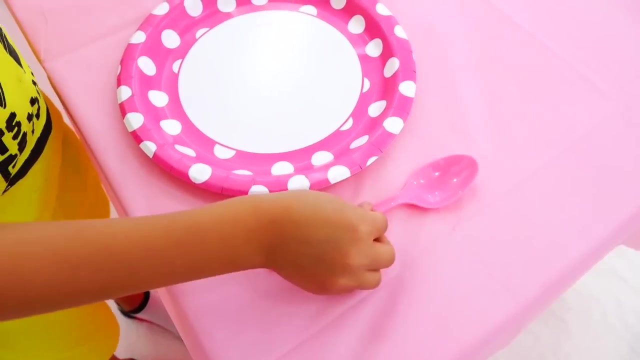 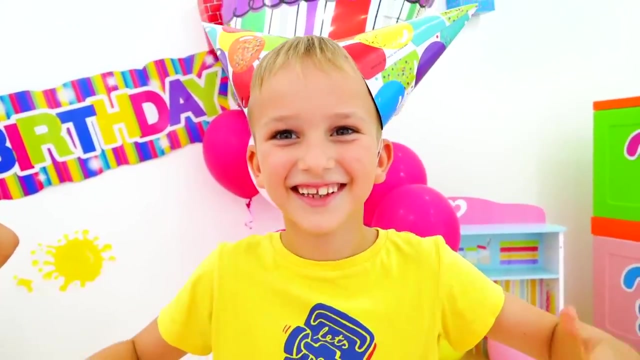 Help. Ooh, Mmmmm, Magic, Better Oops, Perfect Stop For mommy. Yes, Balloosh, Come on, Balloosh, You killed it. Balloosh, Balloosh, Ta-da, Yes, Yes, Yes. 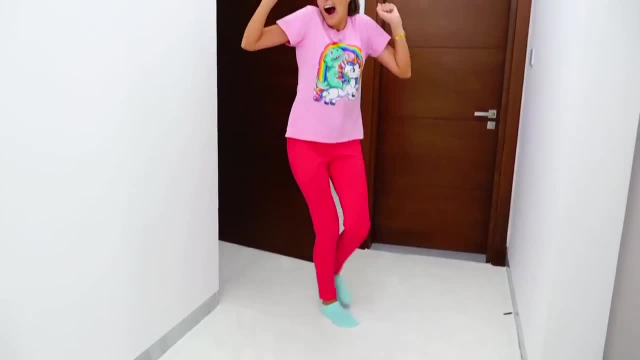 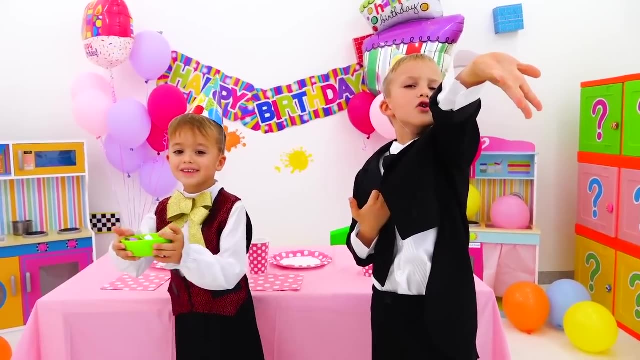 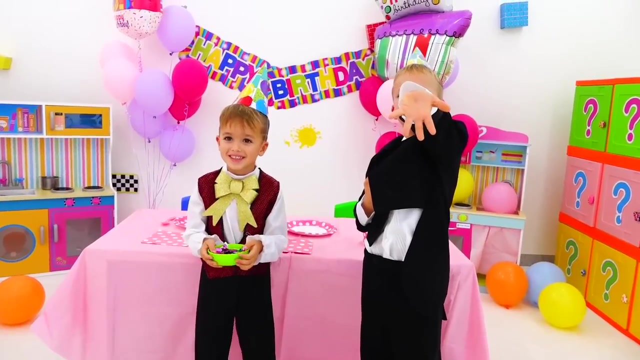 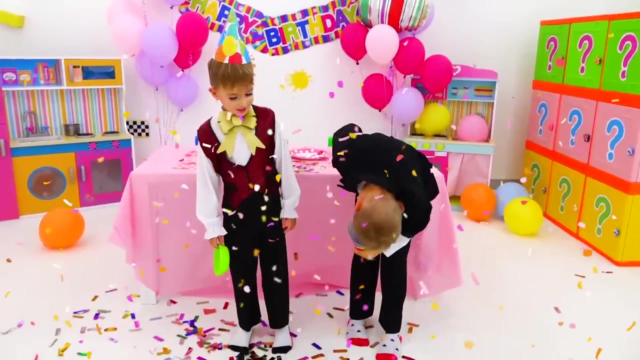 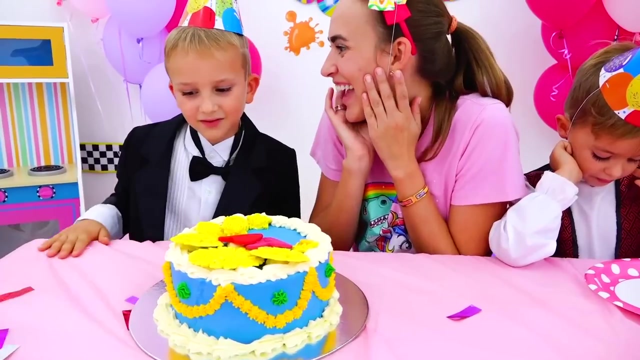 Mommy, Is this for me? Happy birthday to you. Happy birthday to you. Happy birthday, dear mommy. Happy birthday to you. Oh my, This is my cake for you. Thank you, Wow. Here's my cake for you, Wow. 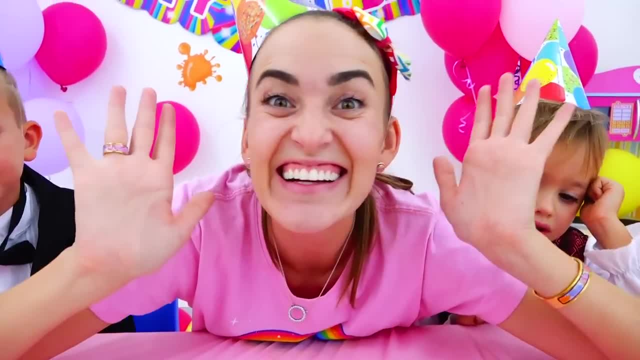 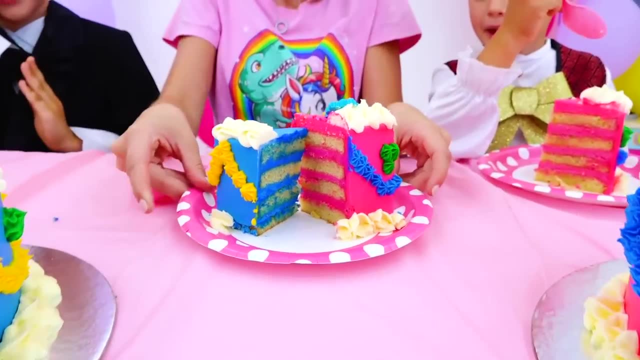 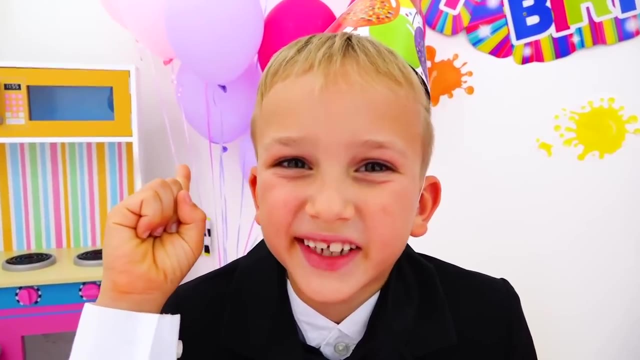 You made it. Let's try. This is for you, Wow, This is for me, Thank you. Thank you, Mmm, Mmm, Mmm. Oh, A present, It's a present from me. Thank you, Wow. 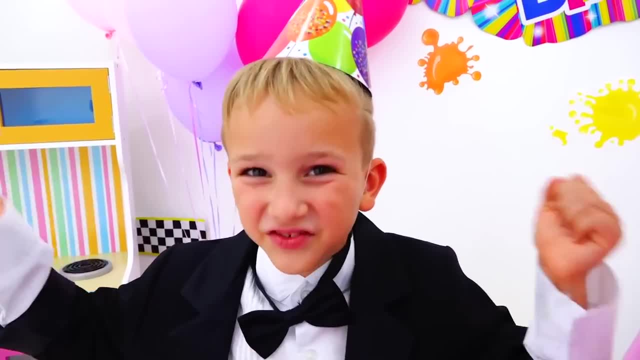 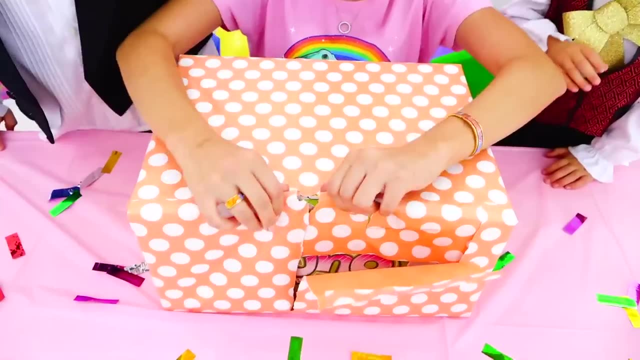 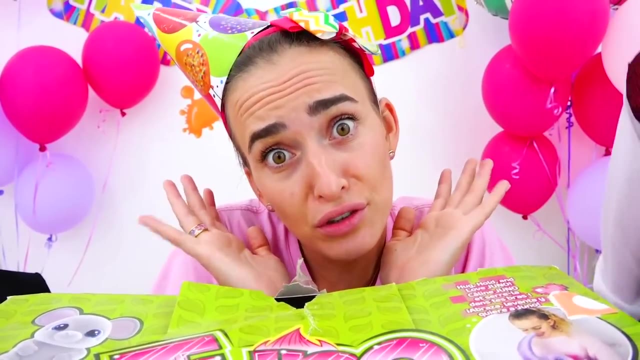 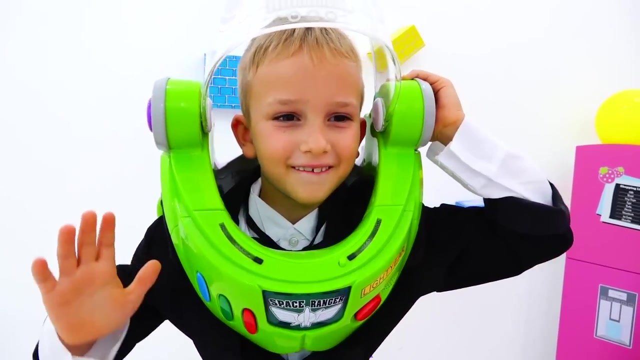 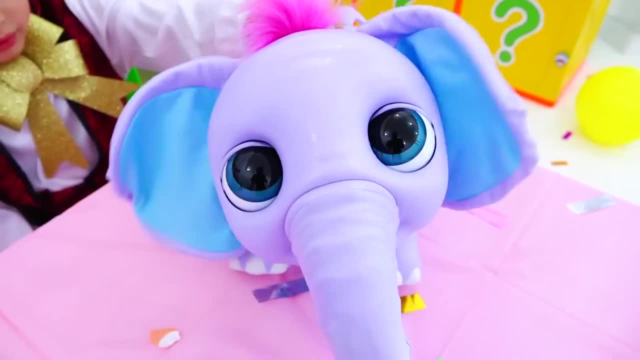 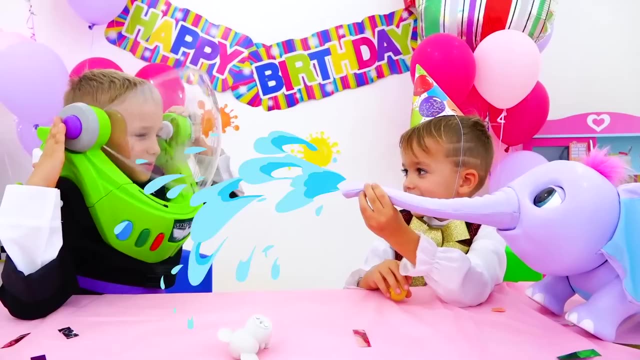 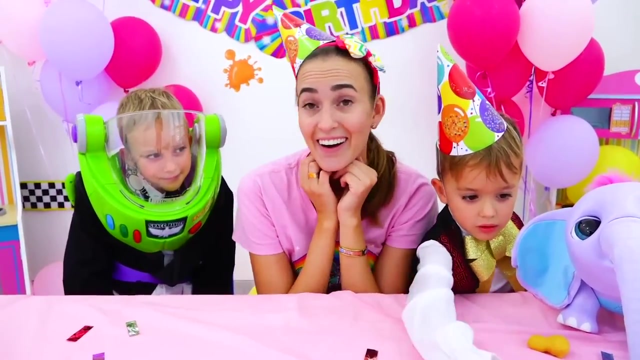 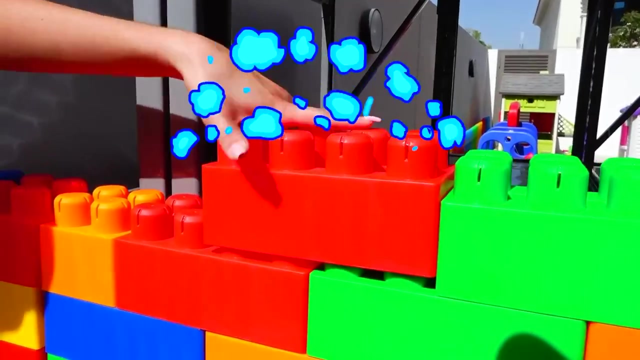 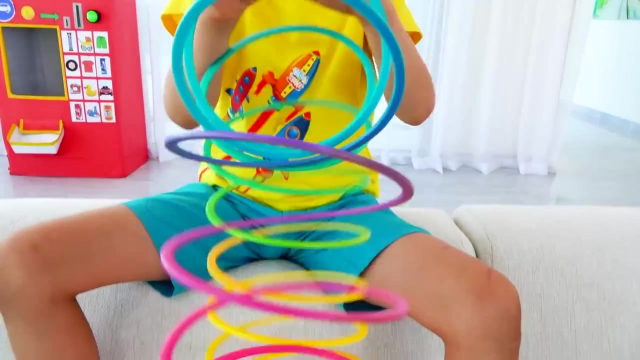 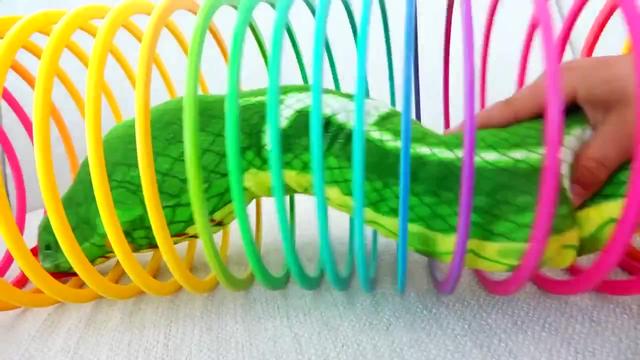 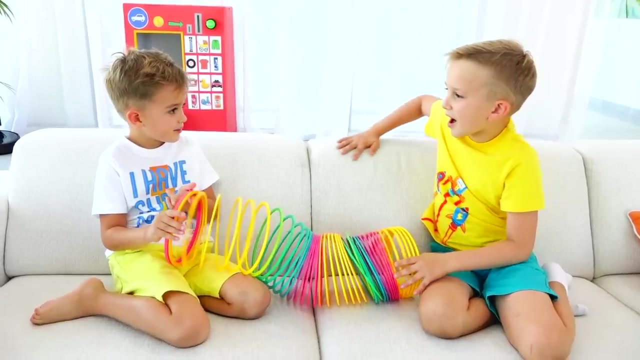 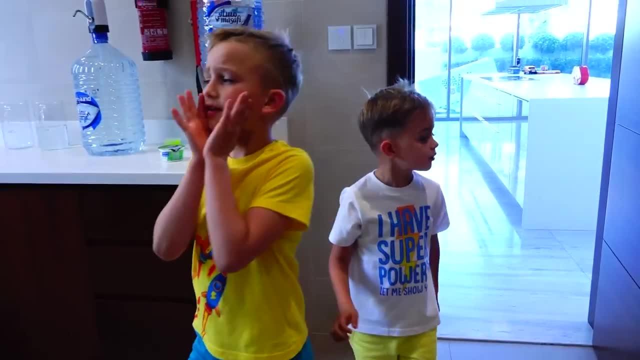 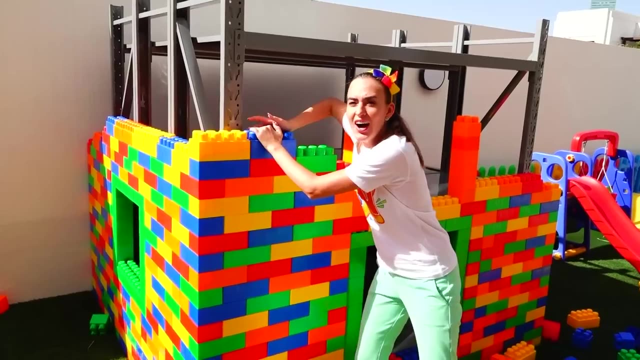 Mommy, Where are you, Mommy? Mommy, Mommy, you're here. Hi boys, Come here and help me. Okay, What are you doing, mommy? I built this three floor house, The house The tiger. 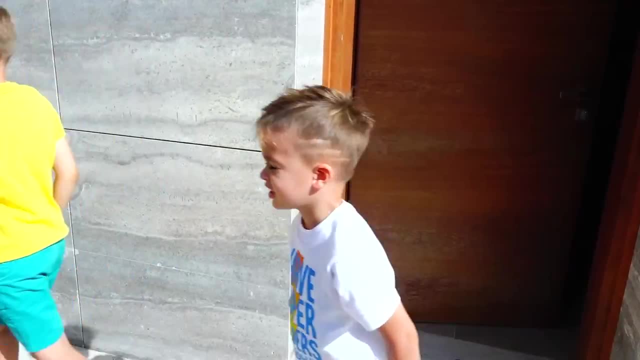 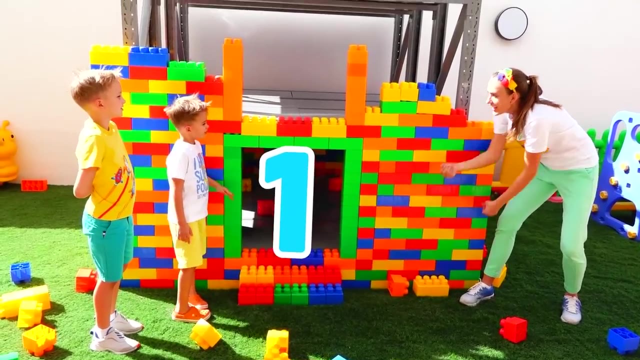 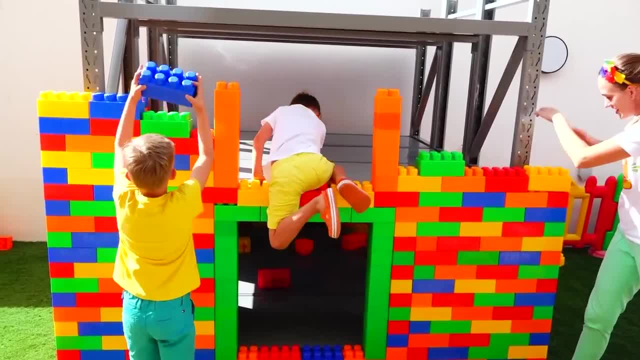 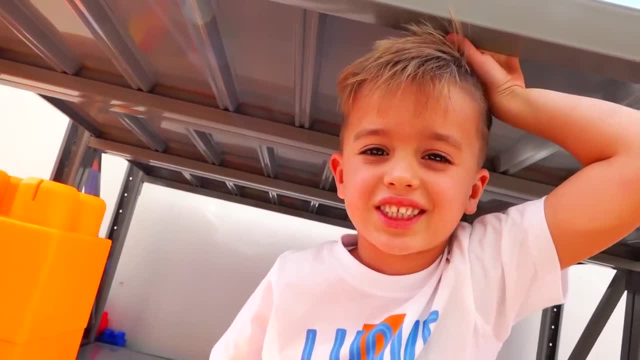 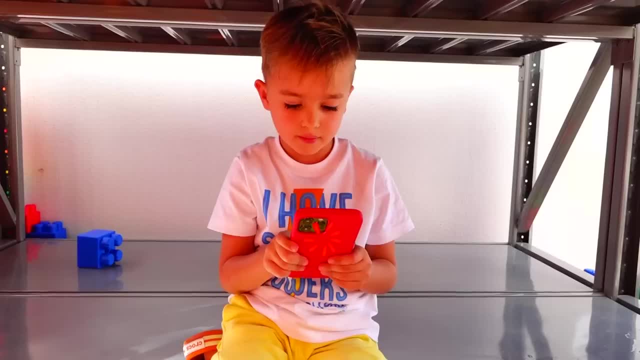 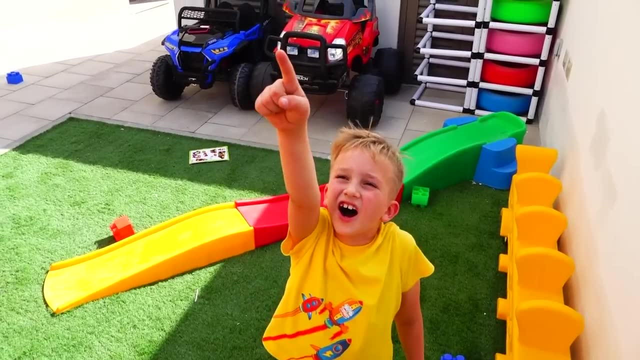 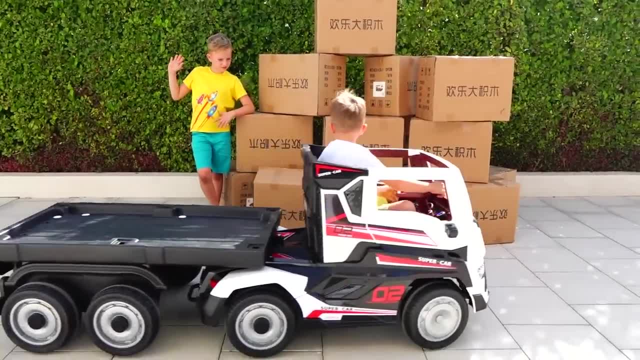 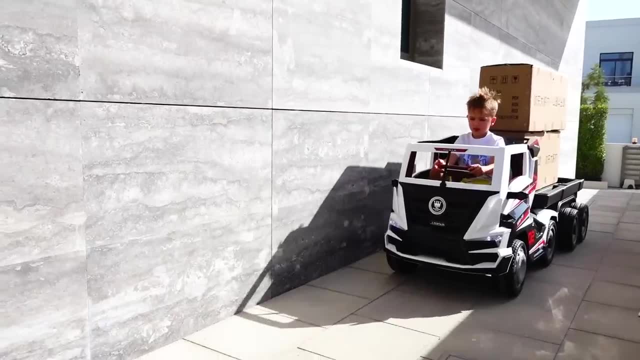 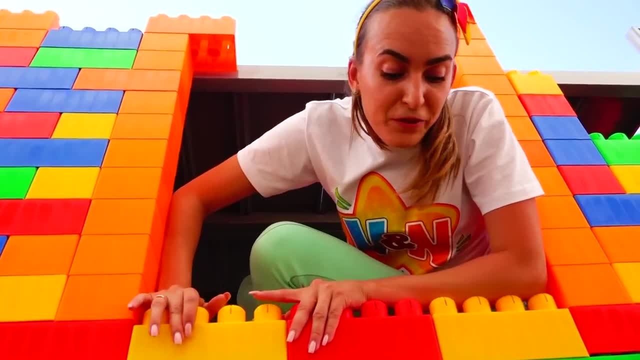 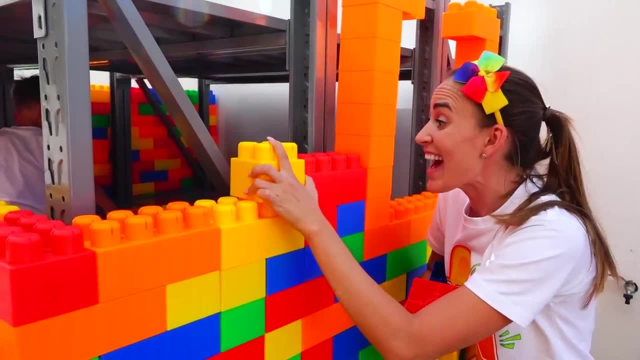 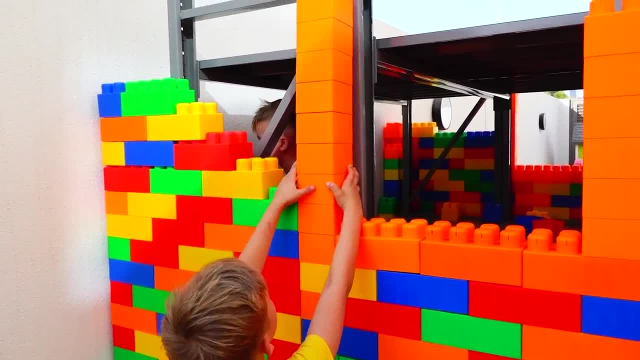 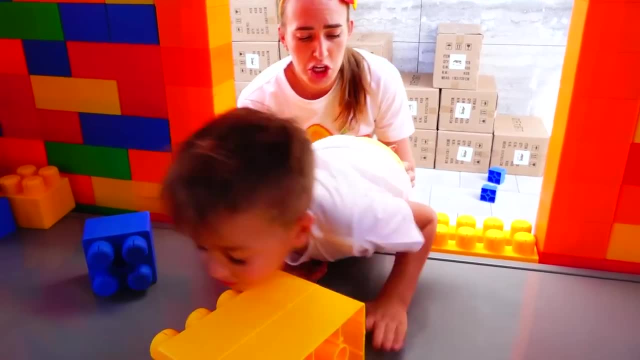 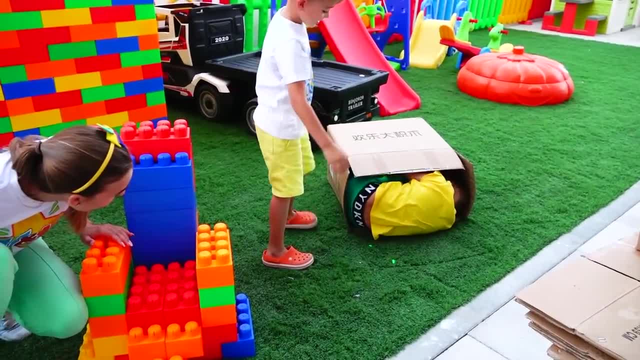 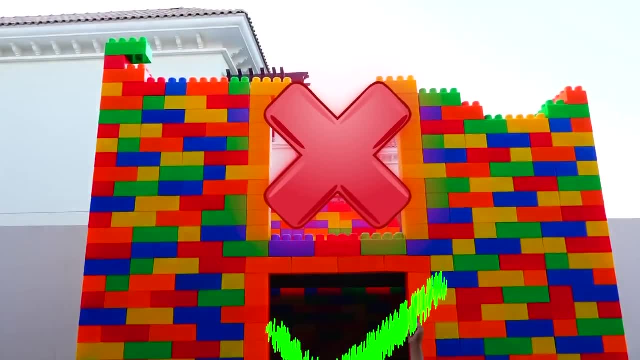 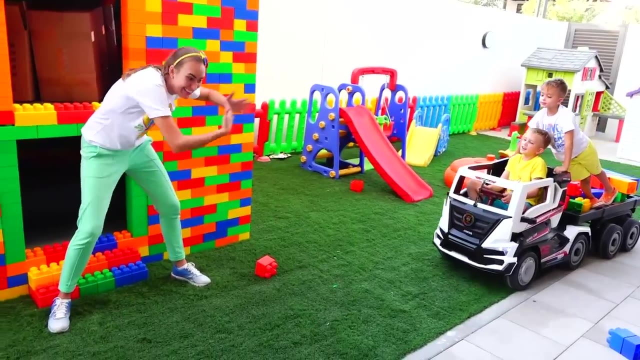 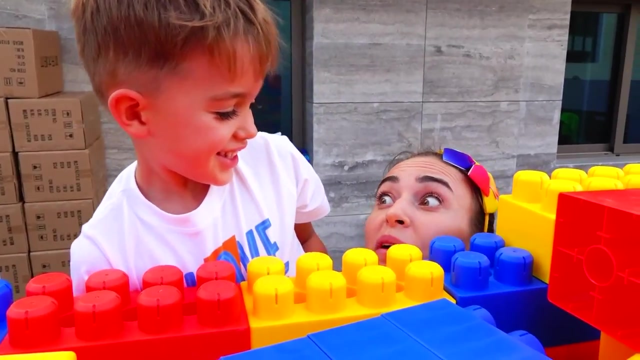 Mommy, Mommy, Mommy, Mommy, Mommy. First floor done, second floor done, third one not done. Come on, Iggy, just go to work. Okay, Oh, yeah, Oh, third floor will be the coolest one. 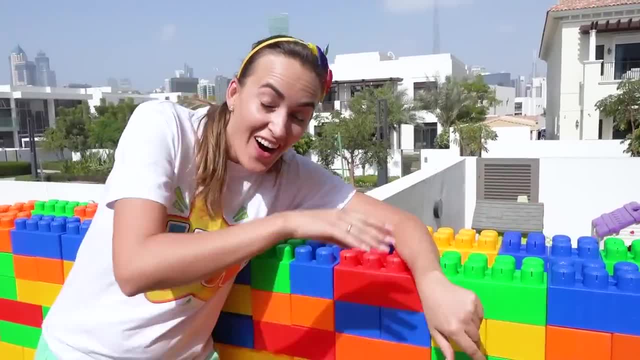 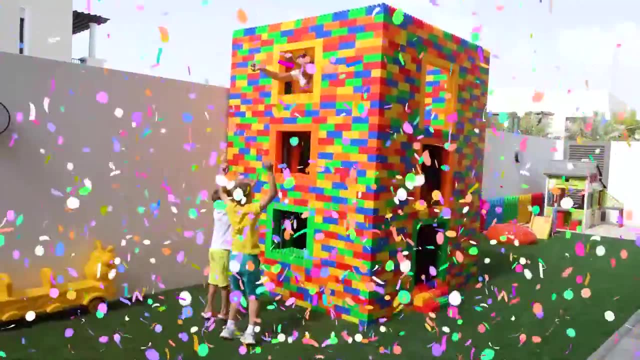 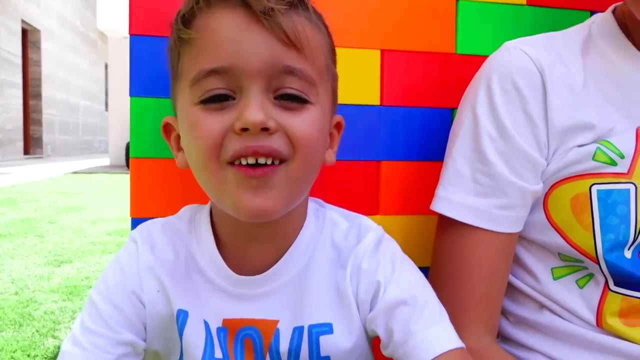 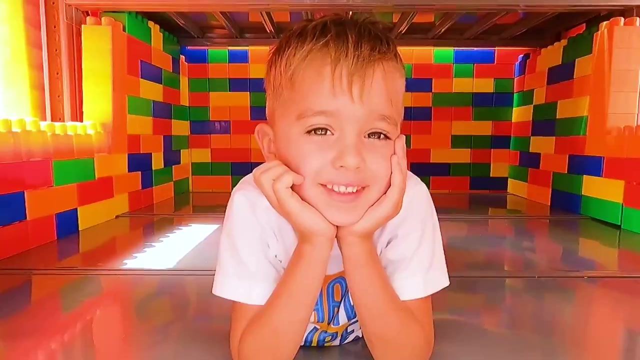 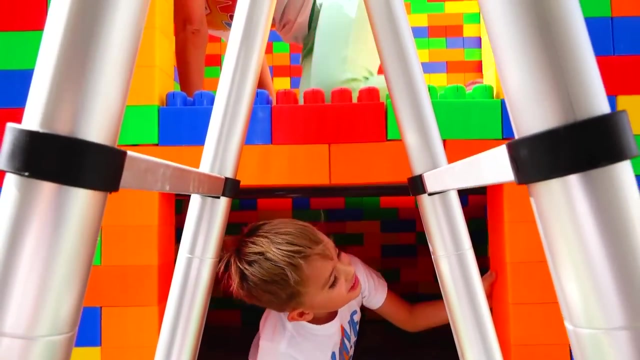 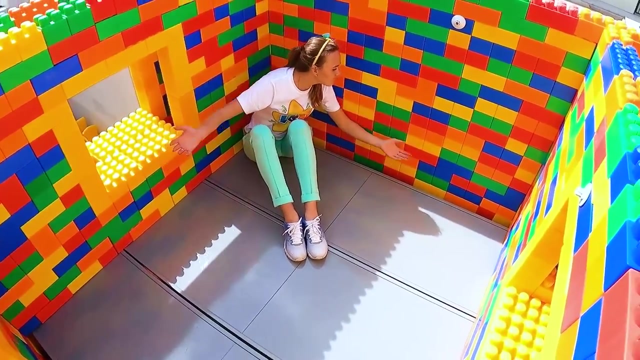 Yes, Finished Boys, our house is ready. Boys, I'm coming. I choose third floor, I want second floor. Okay, I like second floor. Cool, Hi Nikki, Hi Bloss, Hi boys, I'm here. Boys, finish furniture. 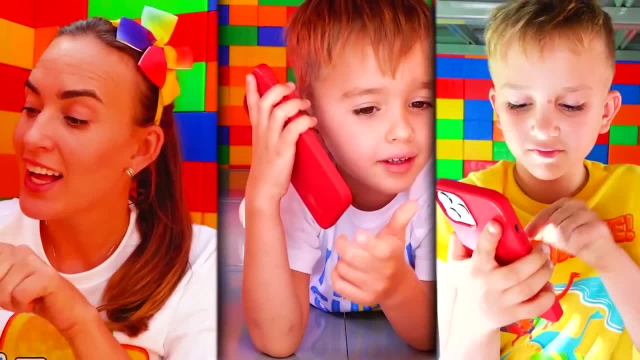 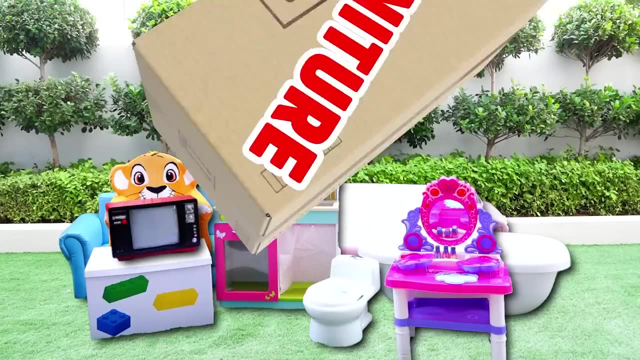 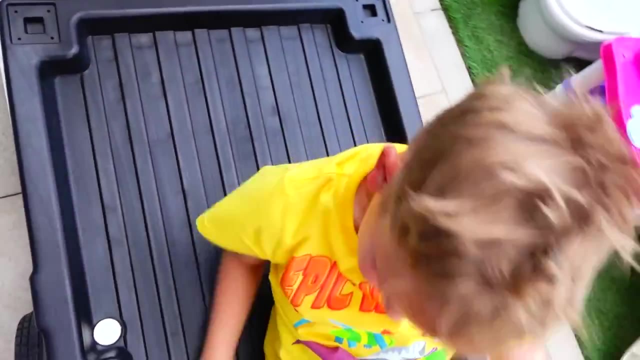 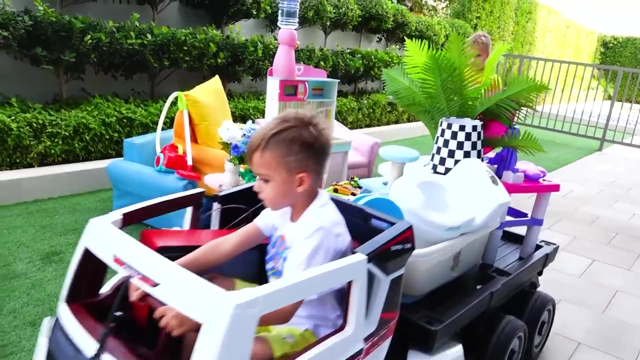 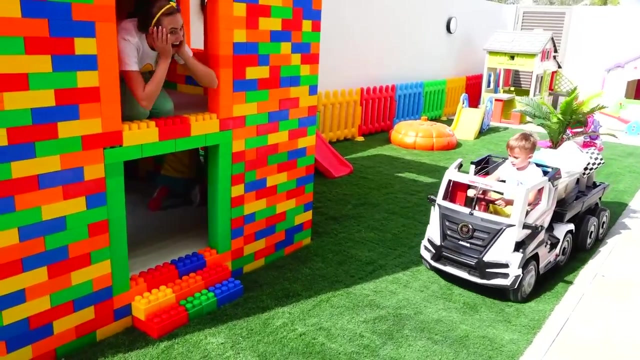 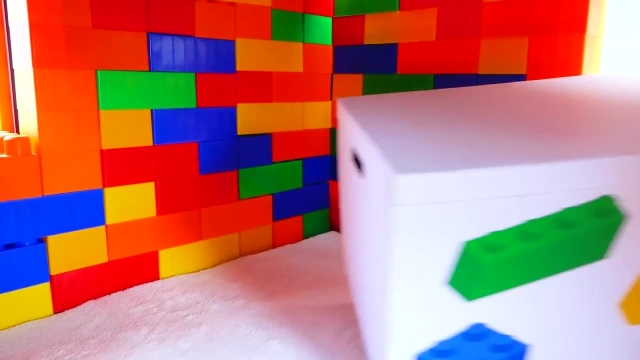 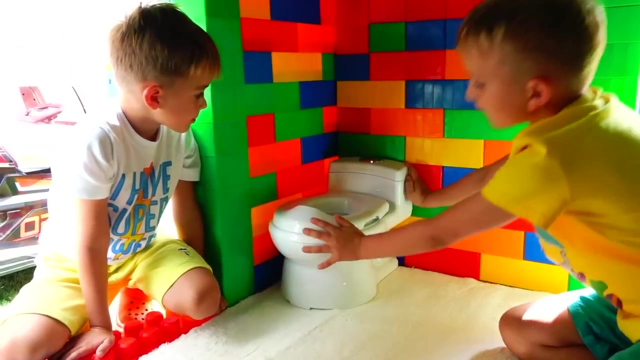 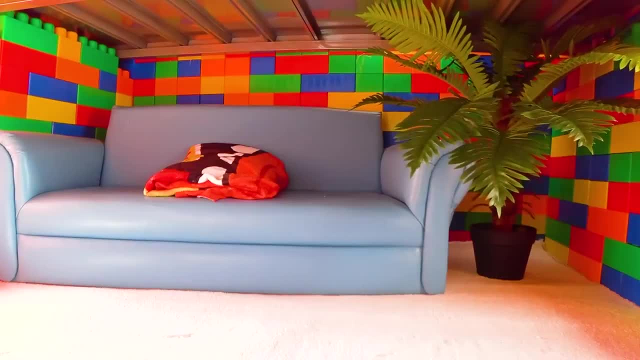 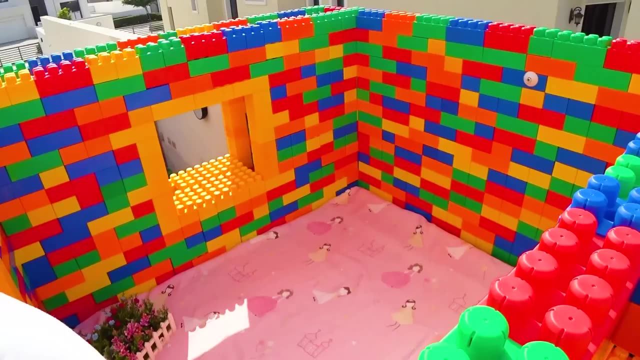 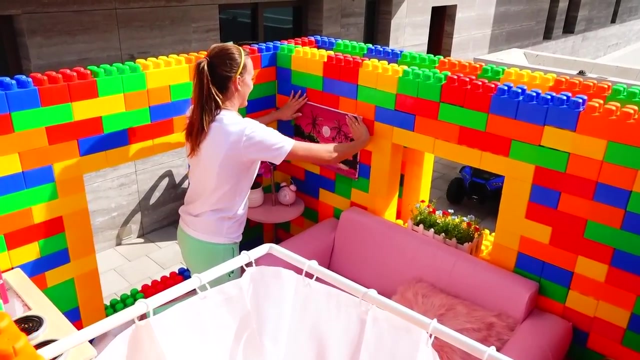 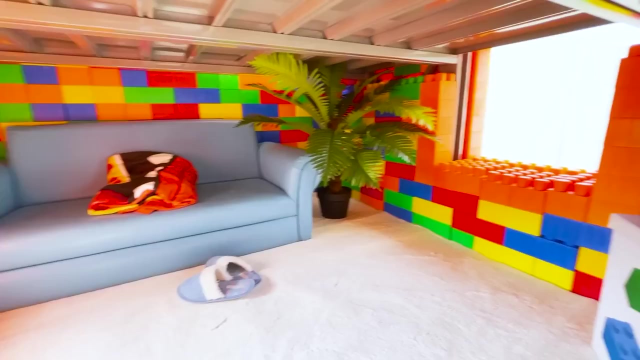 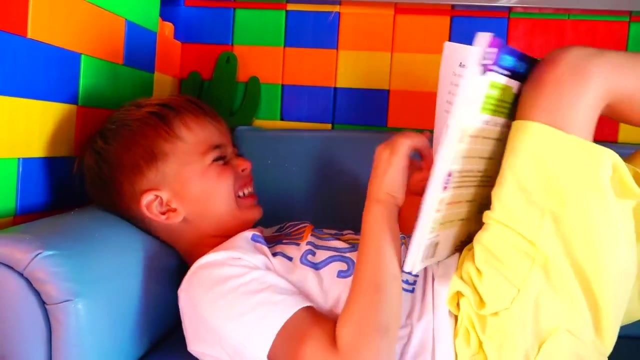 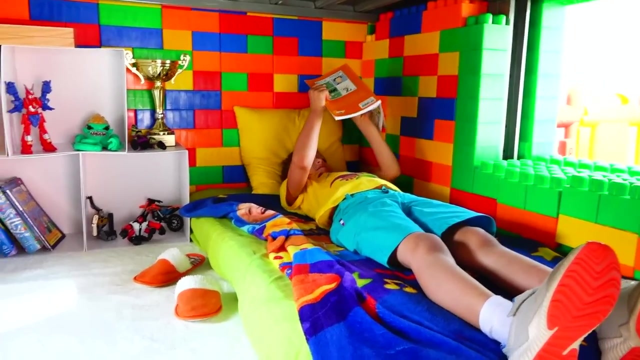 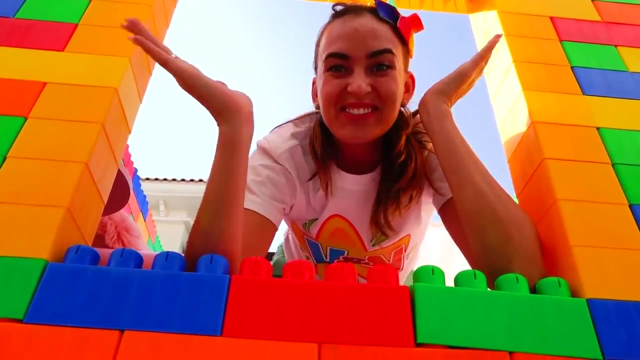 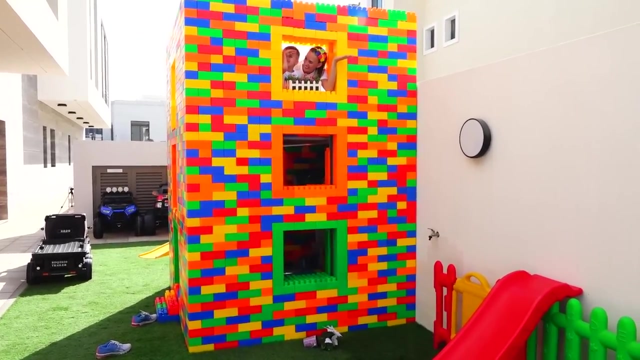 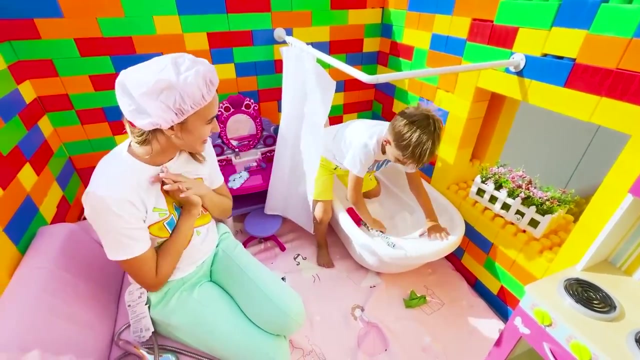 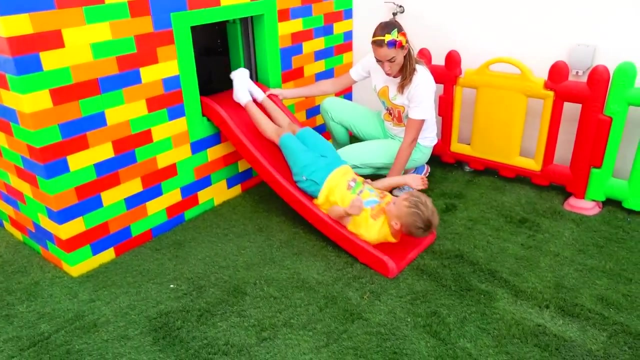 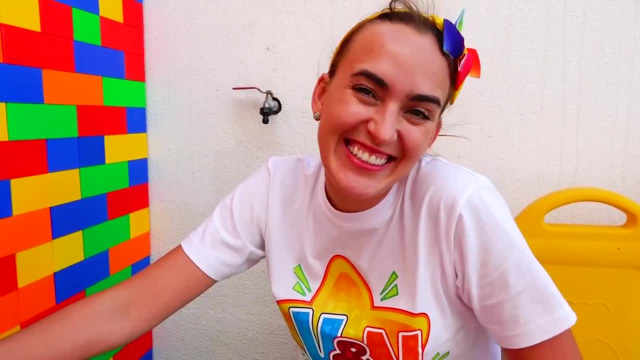 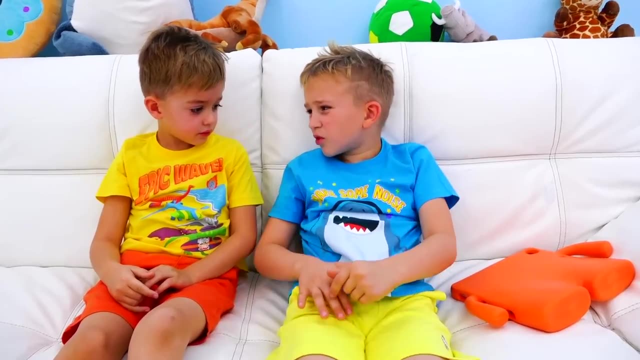 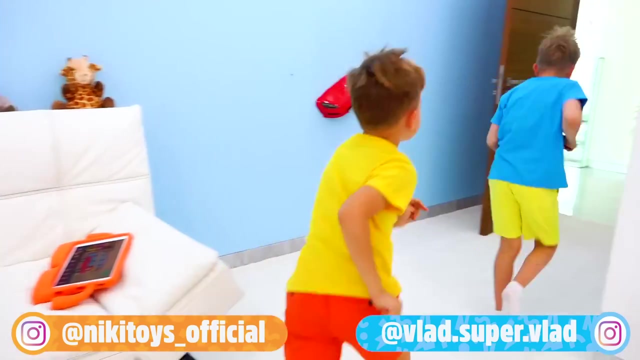 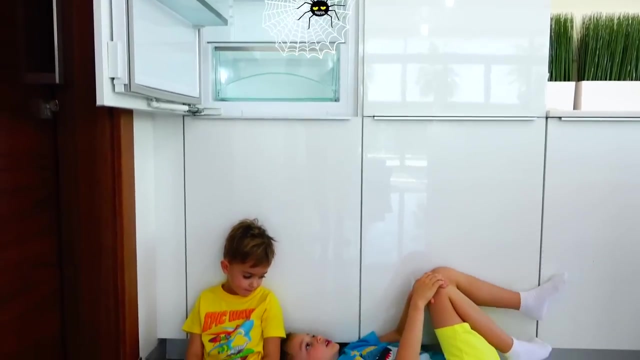 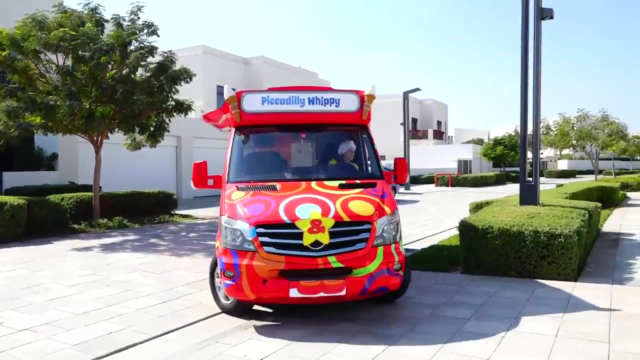 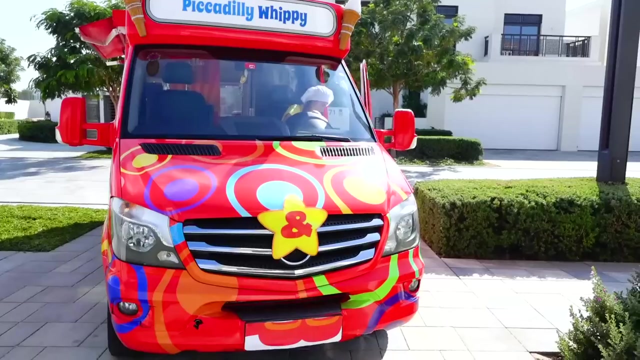 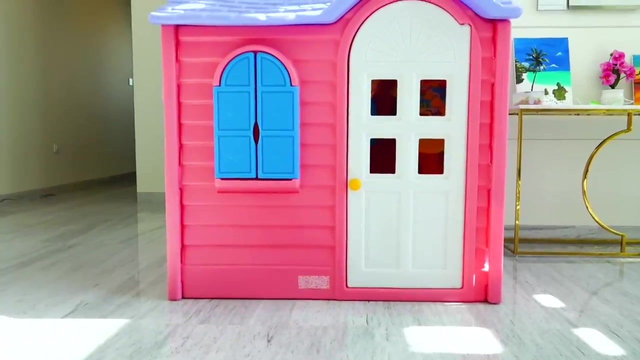 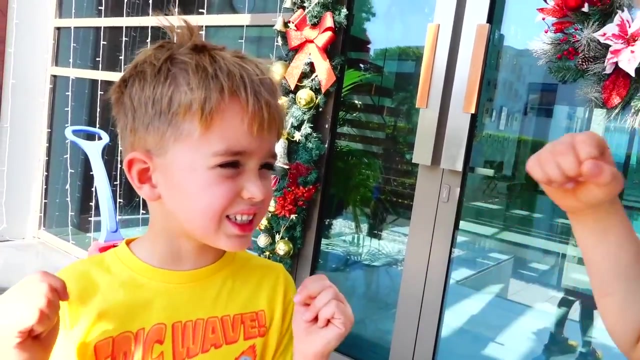 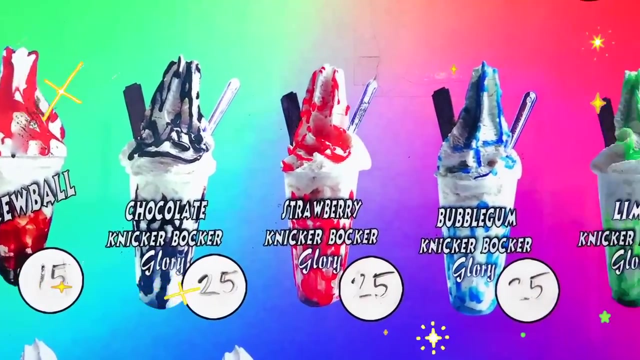 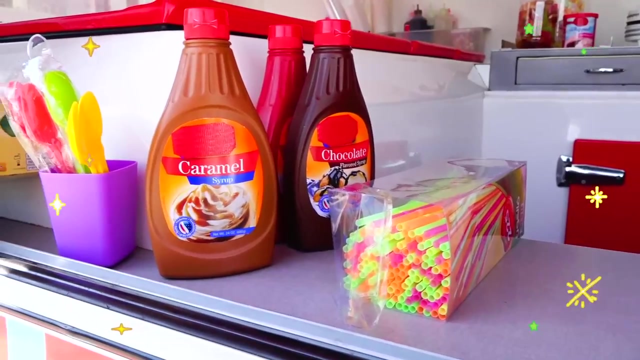 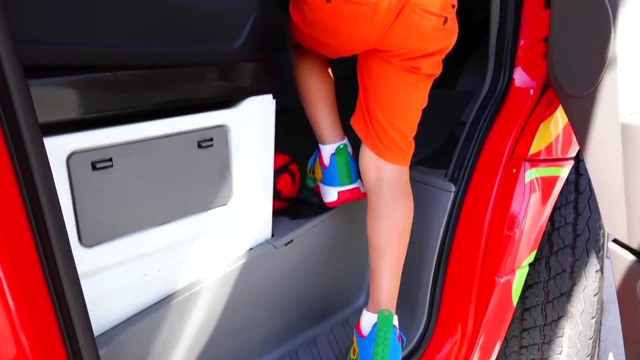 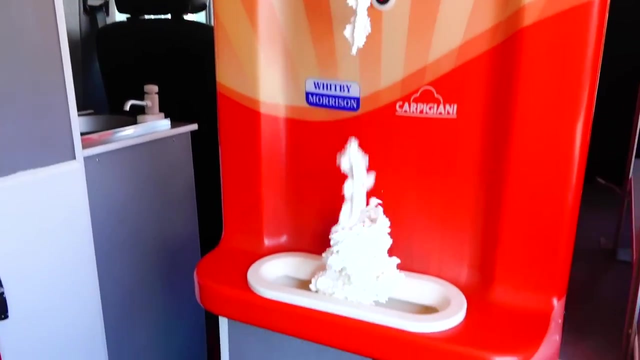 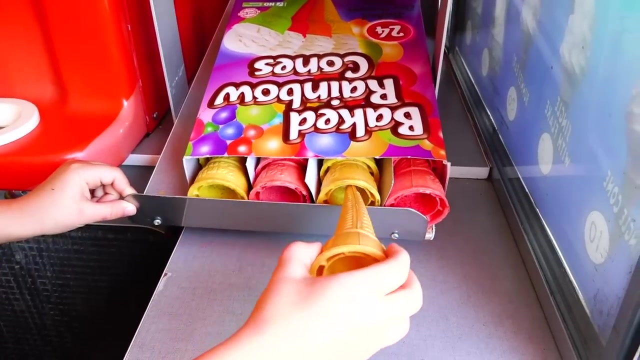 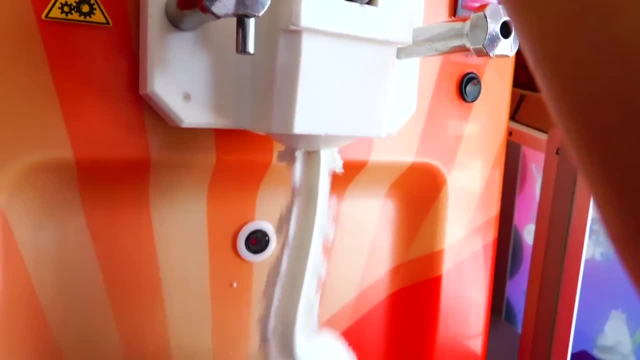 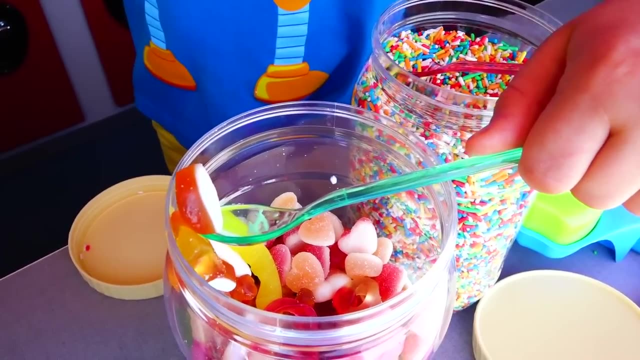 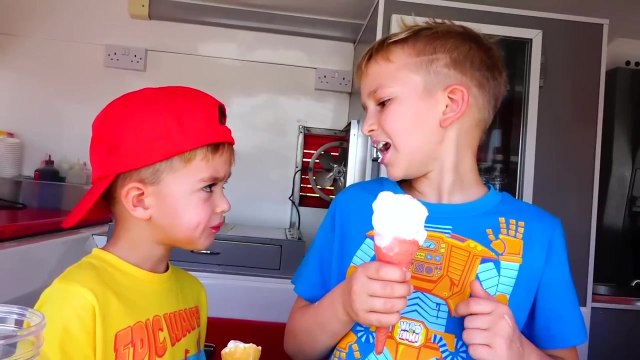 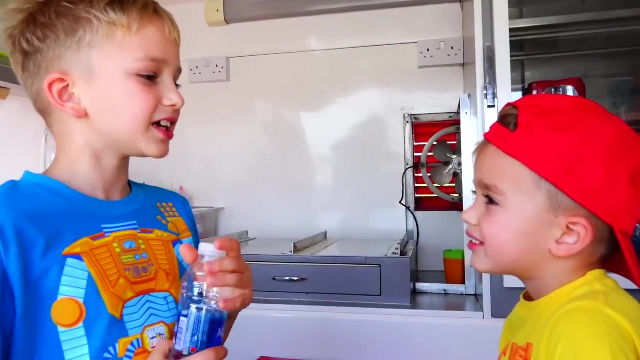 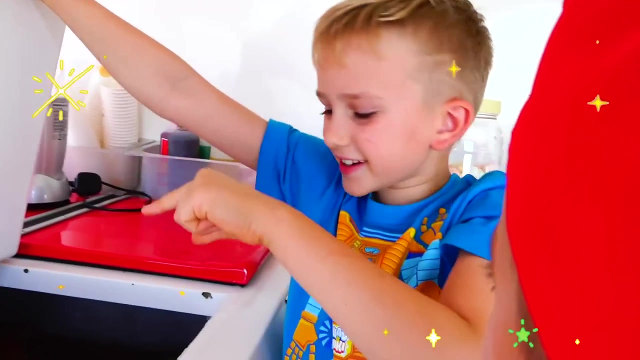 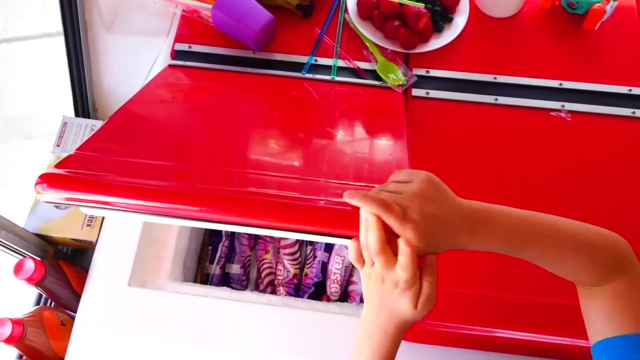 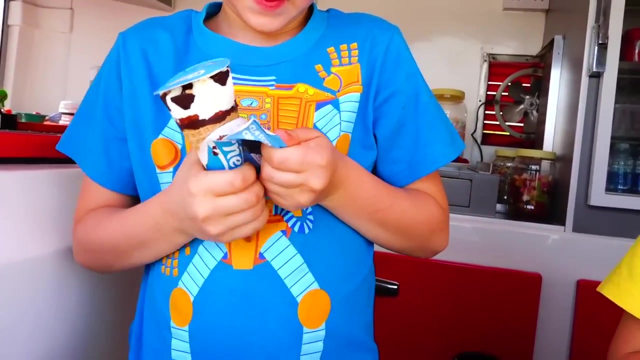 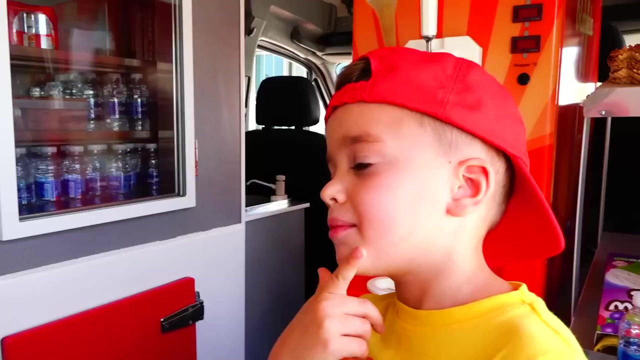 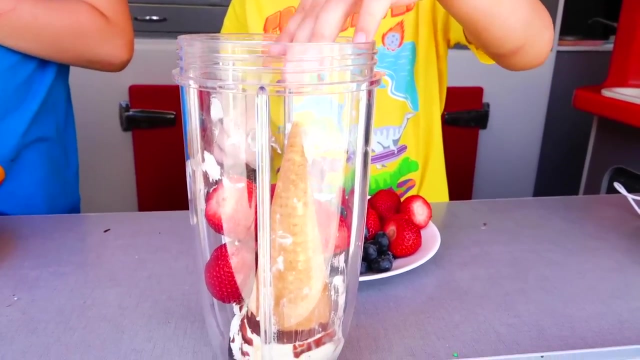 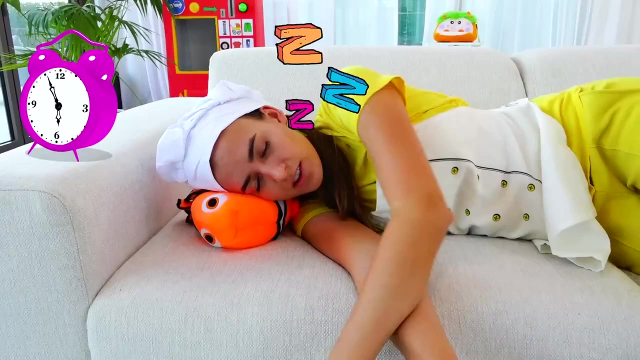 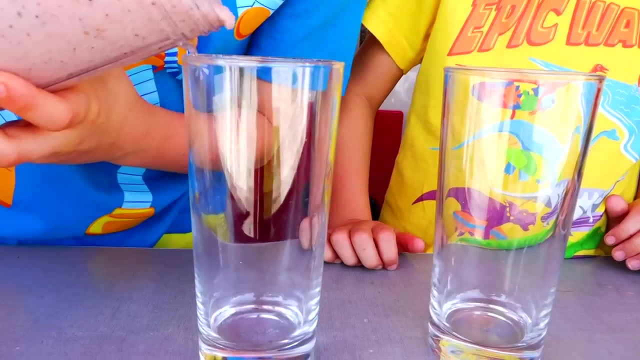 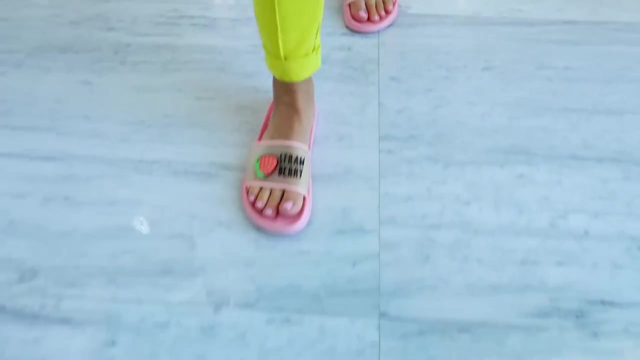 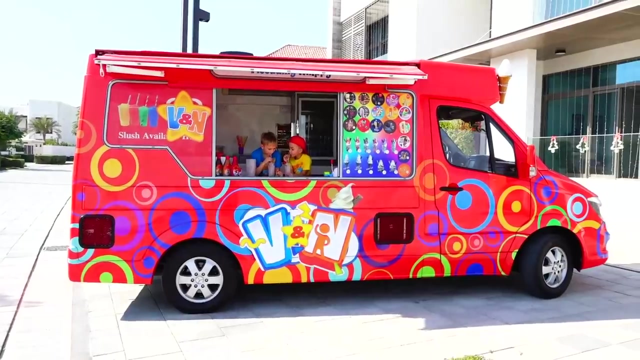 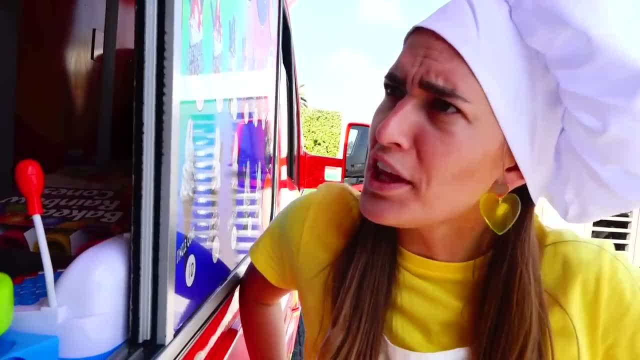 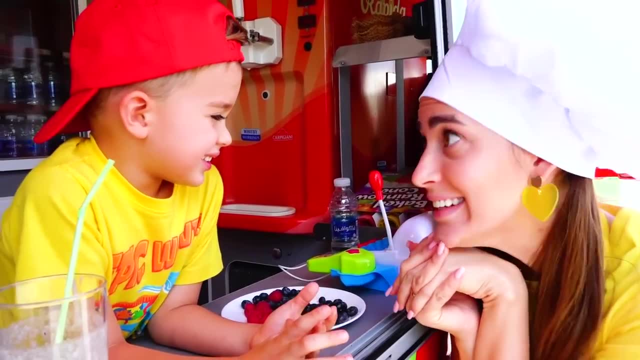 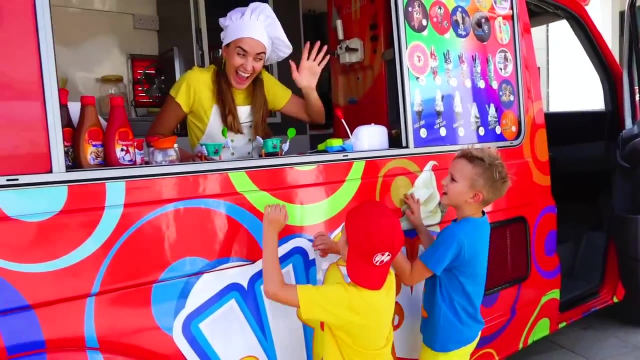 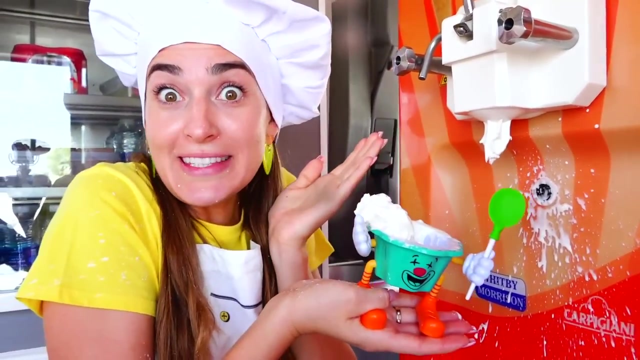 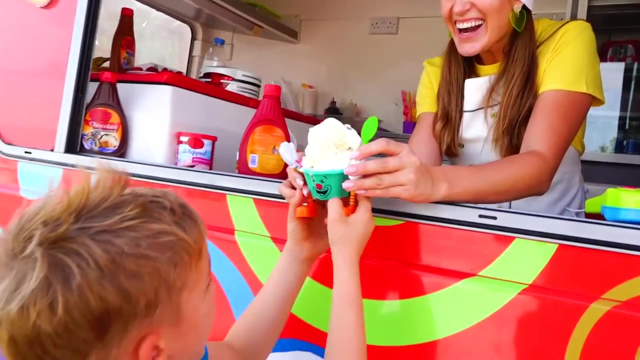 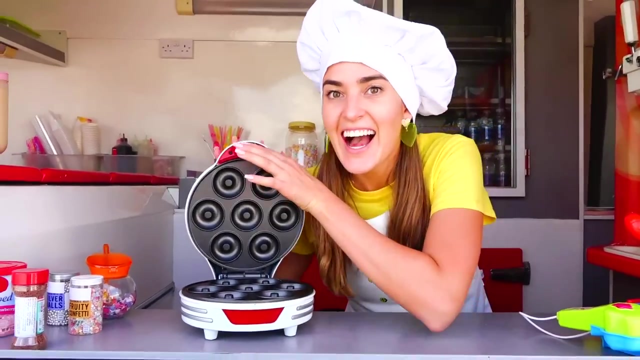 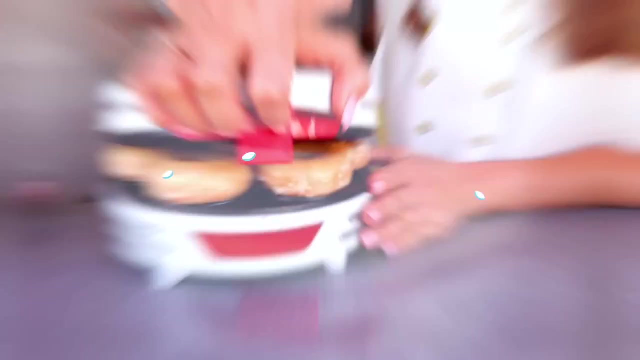 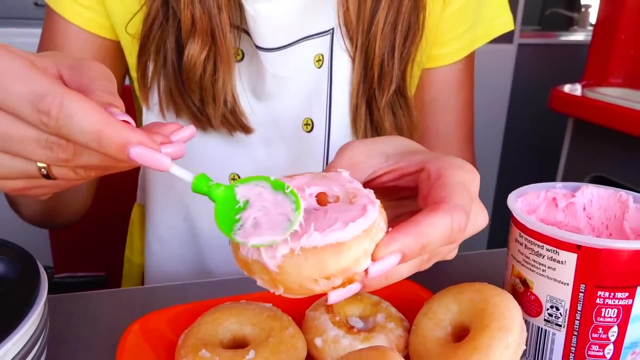 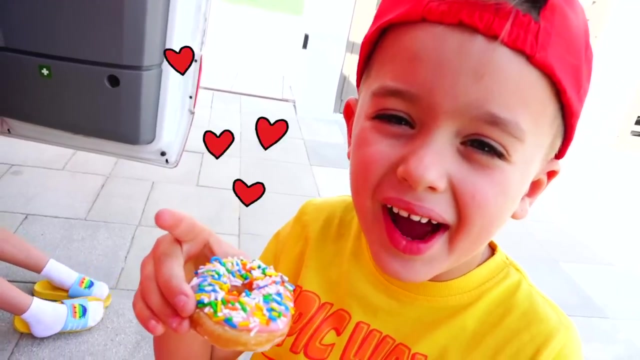 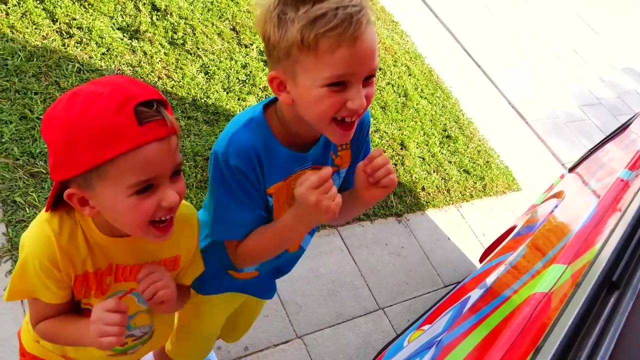 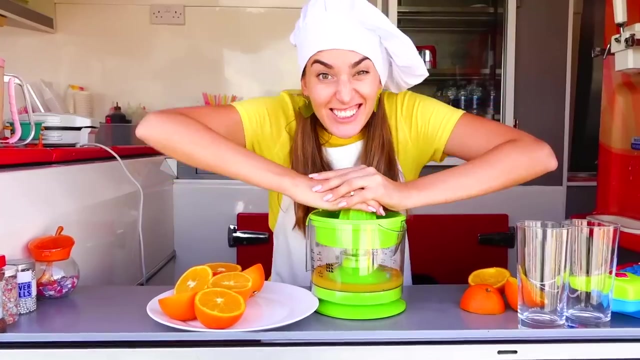 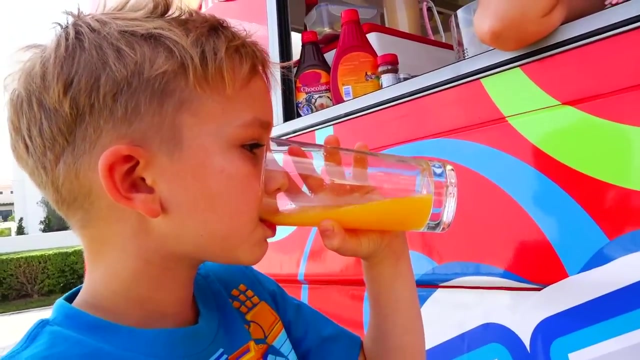 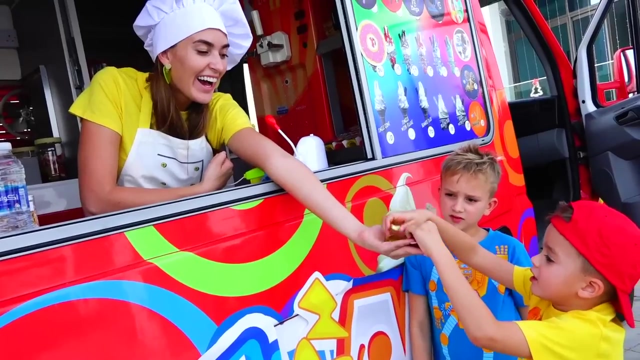 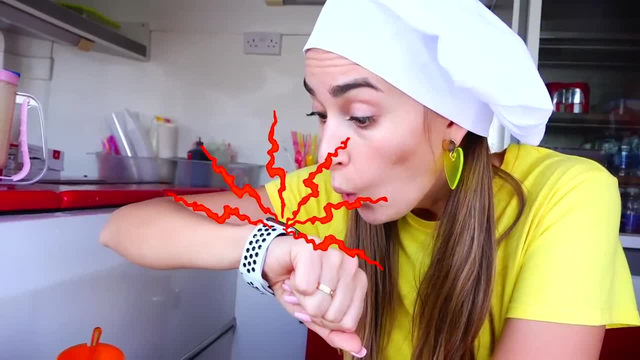 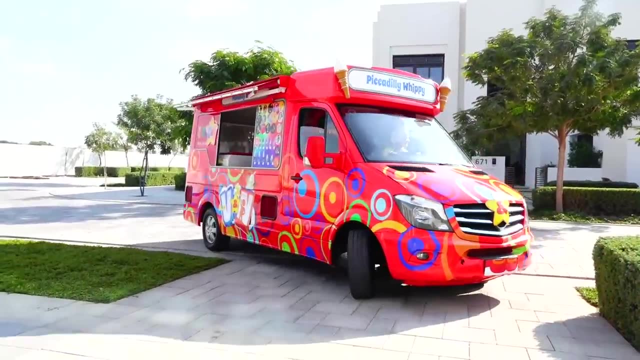